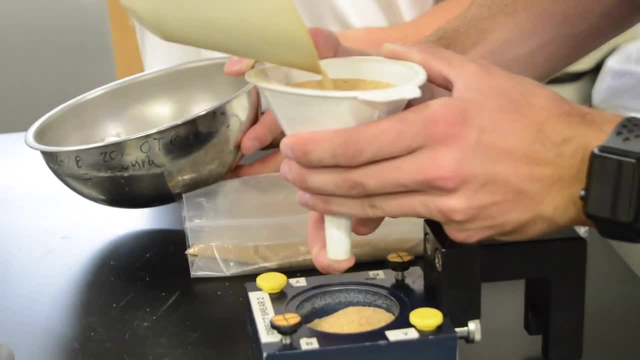 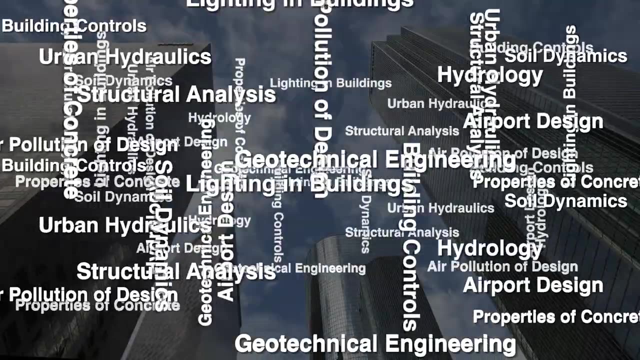 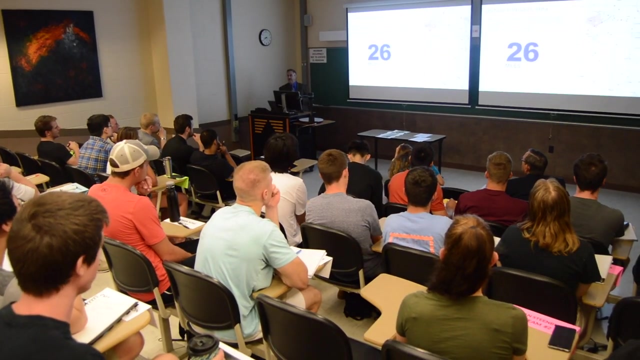 as making and testing concrete samples, testing soil compaction and testing steel strength. In your courses, you'll also have access to over 100 technical electives spanning nine civil engineering emphasis areas. This allows you an incredible amount of flexibility to tailor your 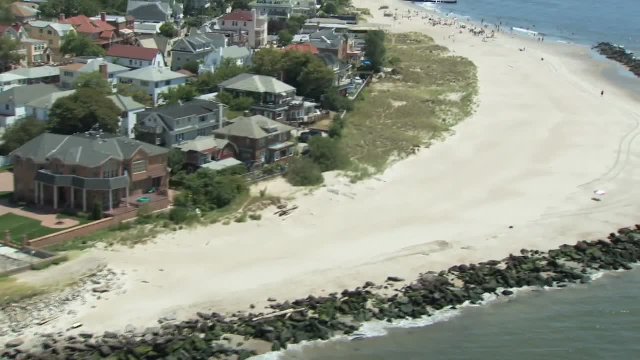 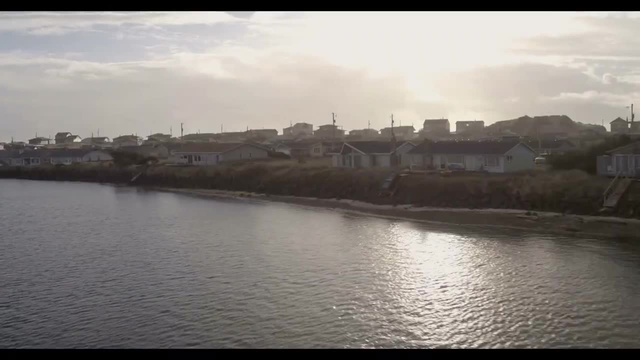 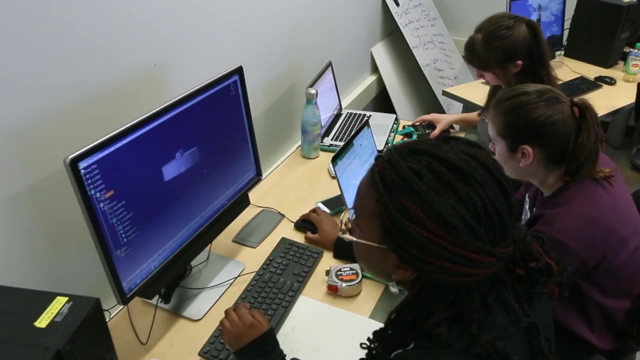 classes to your interests. These courses can include coastal engineering, where you'll study the coastal environment, such as waves, sea level rise and storms, as well as the challenges of building structures along the shoreline. In our Building Components and Systems Design class, you 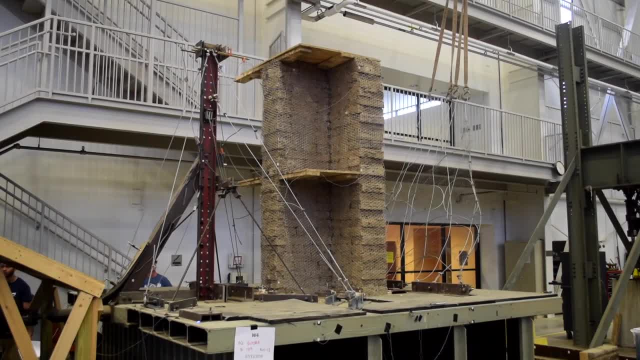 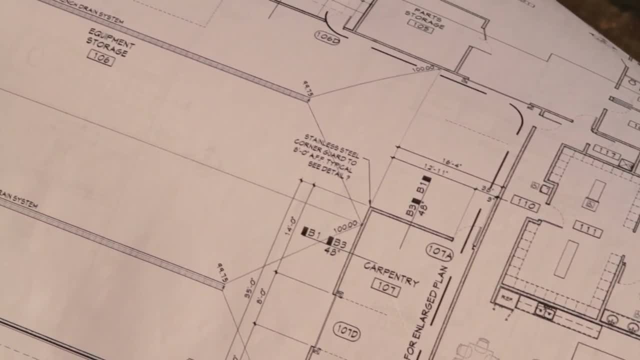 will learn the structural design of a building and how to build structures along the shoreline. You'll also learn about the design process for buildings. This class will teach you about the relationship between architectural and structural drawings, as well as how to design floor and roof systems. 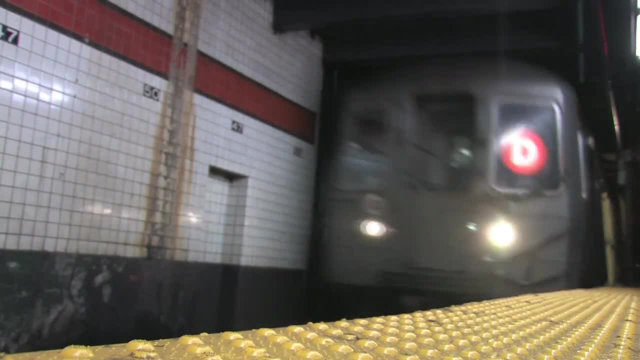 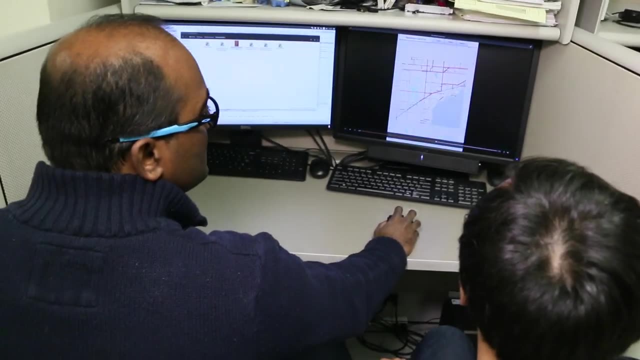 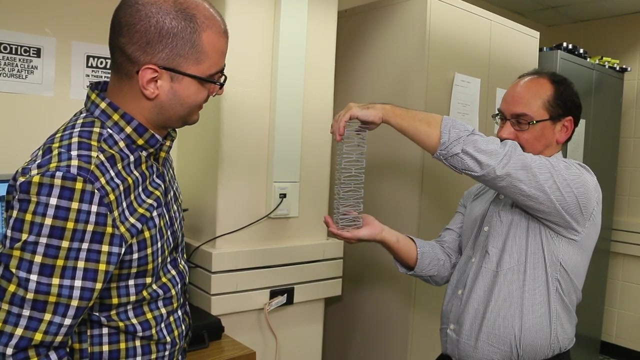 And in our Public Mass Transit course, you'll dive into all things public transit. This interactive class goes over transit funding, scheduling and operations and much, much more. But you won't be alone when you select these courses In your junior and senior years. 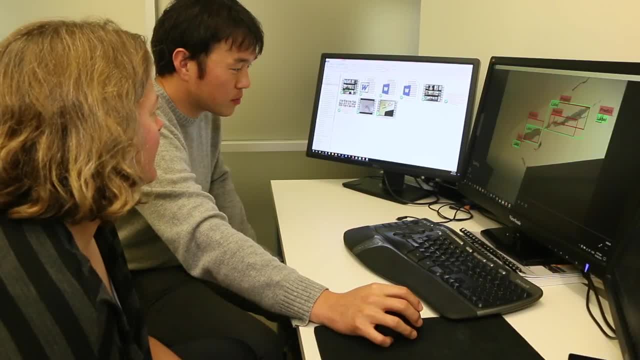 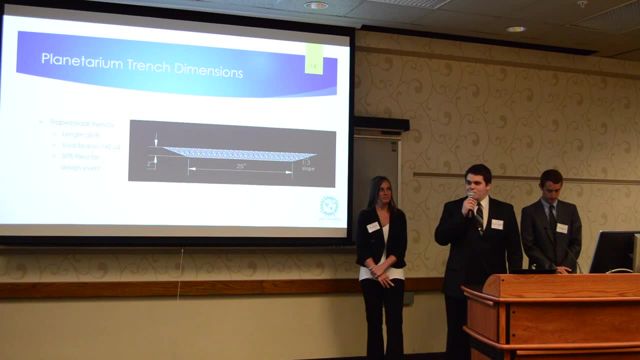 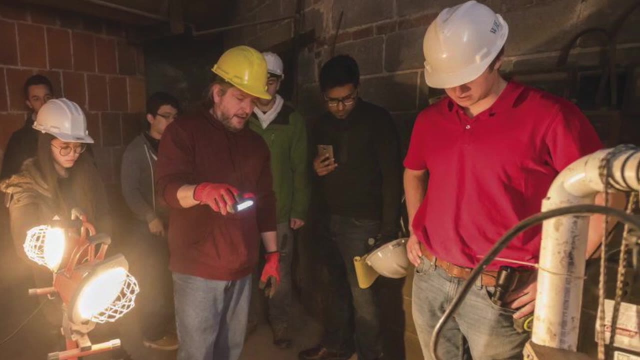 you'll be paired with your own faculty advisors So that you'll receive the best guidance possible in both course selection and academic pursuits. As a closure to your academic career, you'll take part in the senior design course, where you'll work on a real-world project. Past projects have included designing a new soccer, complex upgrading. 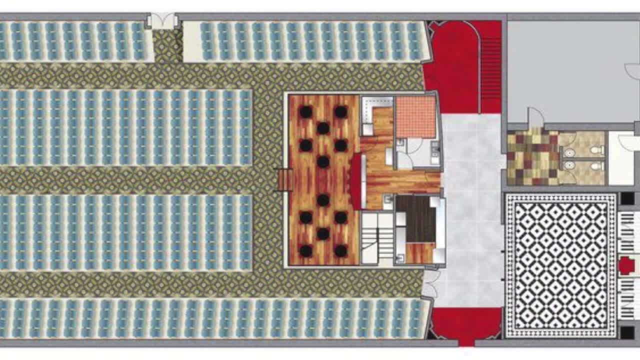 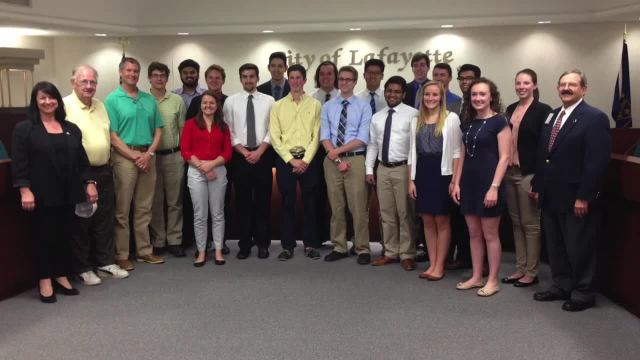 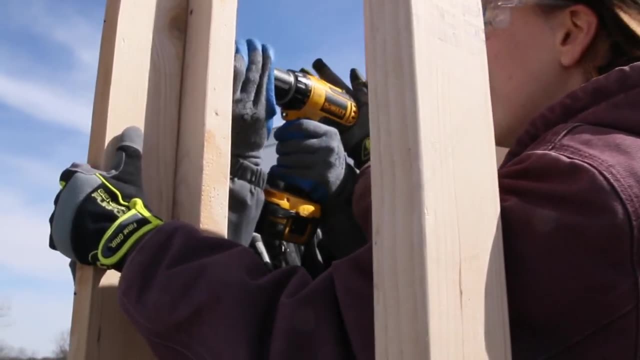 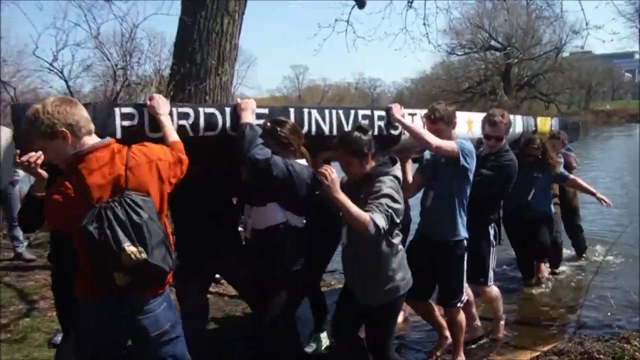 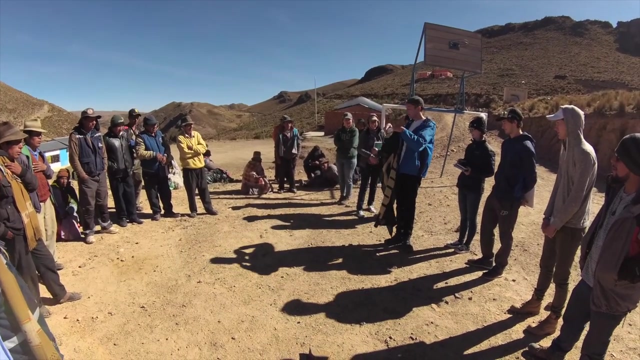 a highway corridor and revitalizing a historic theater. In senior design, you'll be split into teams, tackle different facets of the design process and learn how to build structures along the shoreline. By completing a course, you'll be able to work on building an inclusive auditorium and dark removal studios. You'll be able to work on building an interior design project and communicate your final plan to industry and government officials. You'll also have plenty of chances to participate in our student groups and their activities. One notable project includes a canoe race, where students design and build a canoe made out of concrete and race it against other universities. You can also travel the world and help communities gain better access to vital resources such as clean air and watersten air and water.